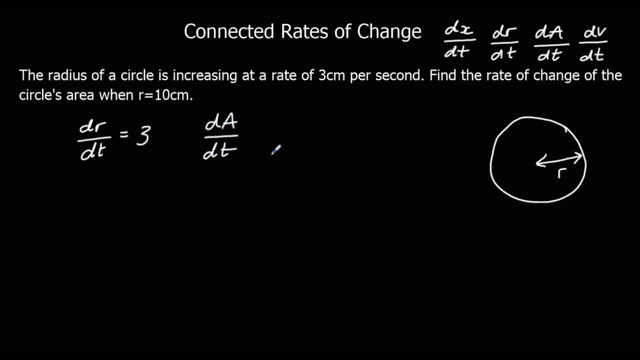 the rate of change of the area. so da dt when r is 10.. So how are we going to find da dt? So whenever we talk about connected rates of change, we're going to be using the chain rule, So we're going to say da dt is going to be da d something. 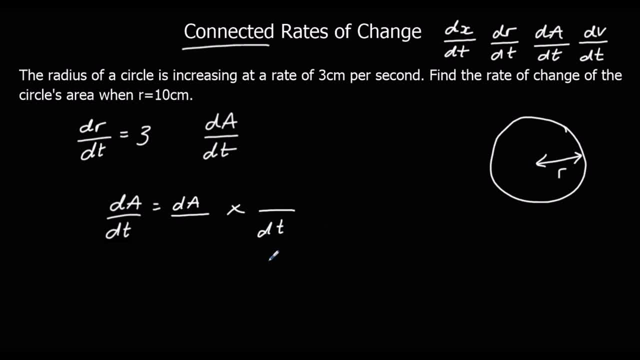 So we're going to have the same variable in these two and they're going to cancel out. So what variable are we going to put in them? Well, there's only one other variable in the question, and that's r, And we already know dr dt. So we'll have dr dt here and here. 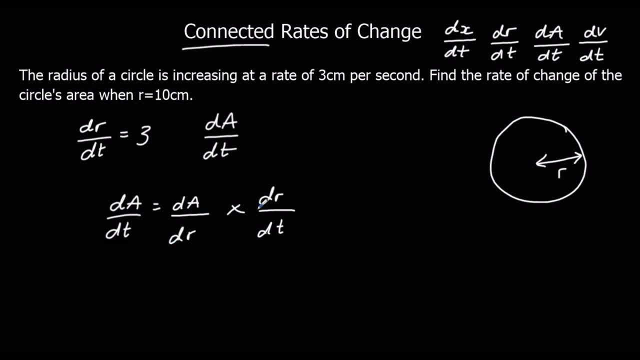 we'll have da dr, And then you can think of the drs as cancelling out, leaving us with da dt. So we know dr, dt, which is 3.. We don't have da dr, So do we have a formula that links? 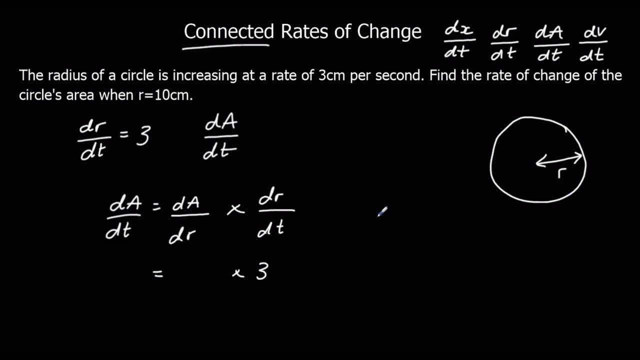 a and r. Yes, we do. For a circle a is pi r squared, So we can find da dr by differentiating with respect to r, So da dr times by the power. Take one off the power, We've got 2 pi r. So da dt is 2 pi r times 3.. So we'll simplify. 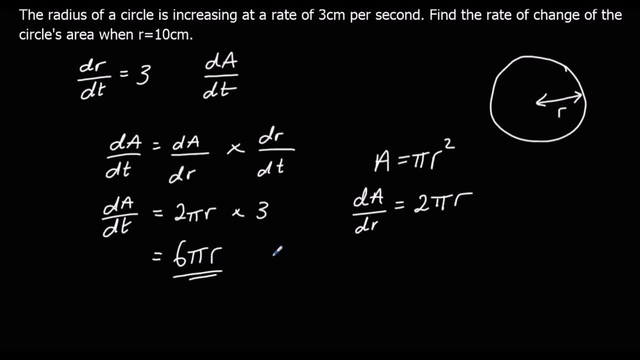 that to 6 pi r. We want the rate of change when the area is 10, when r is 10.. So when r is 10, when r equals 10, the a dt, The a dt is going to be 6 pi times 10, or 60 pi. 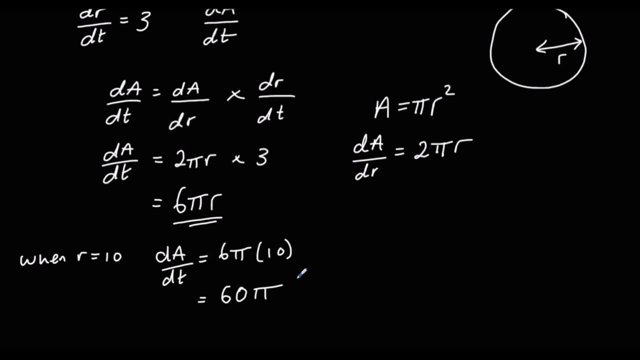 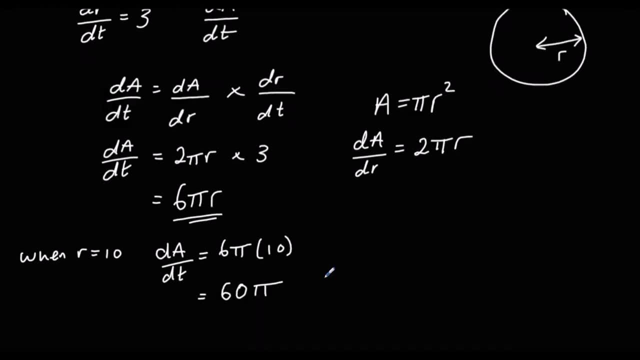 How about the units? So it's the rate of change of the area And the area. well, the length was in centimetres, So the area is going to be centimetres squared And the rate of change per second. So 60 pi centimetres squared per second. 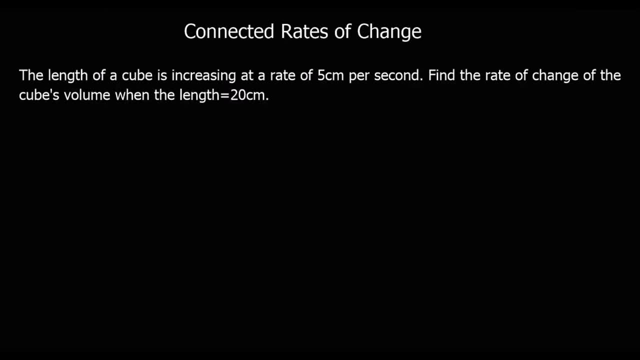 second. okay, here's another question. you could pause the video, try and give it a go or keep watching and i'll go through the answer. so we've got a length of a cube is increasing at a rate of five centimeters per second, so this time we've got a cube. 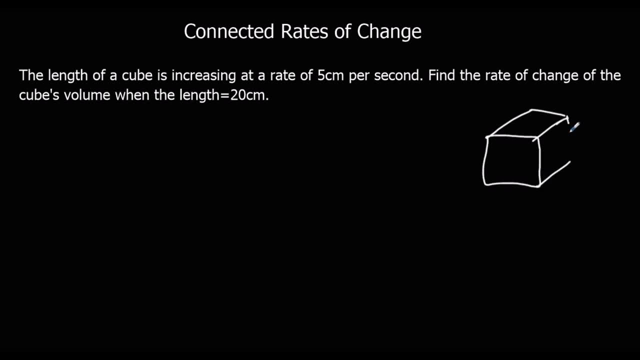 we've got length, so it's a cube. so all the all three measurements here are the same. the length is increasing at a rate of five centimeters per second. so the rate of change of the length dldt is five. so the cube's getting bigger and bigger. 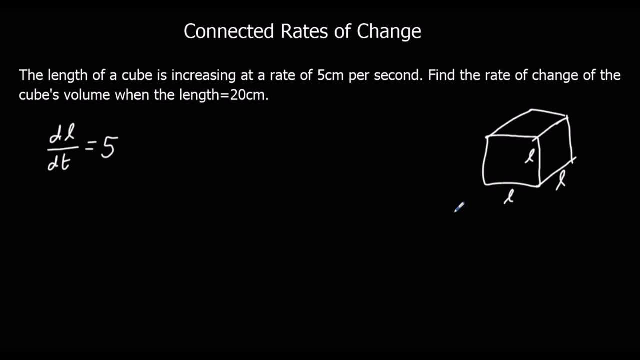 and the length is growing at five centimeters per second. find the rate of change of the cube's volume when the l is 20. so we want dv dt, the rate of change of volume, dv dt, and that's going to be dvd, something times d, something dt, and we're going. 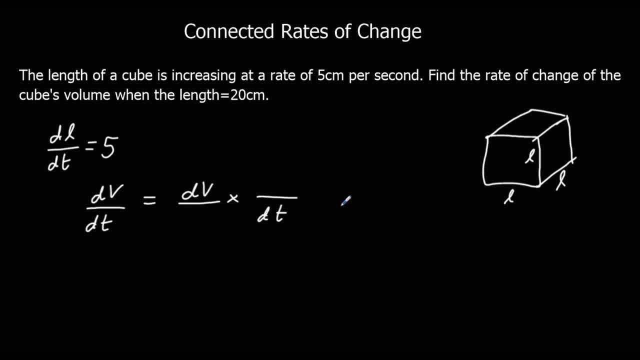 to use l, because that's the other variable that we've been given in the question. so we're going to have dvd l times dl, dt. we already know dldt, that's five. how about v and l? what formula links v and l? so the volume of a cube is the length cubed, so dvdl. 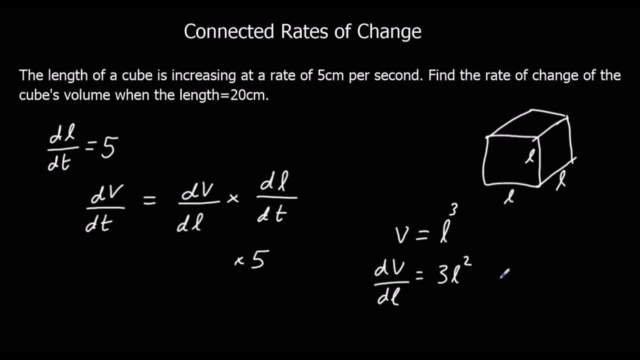 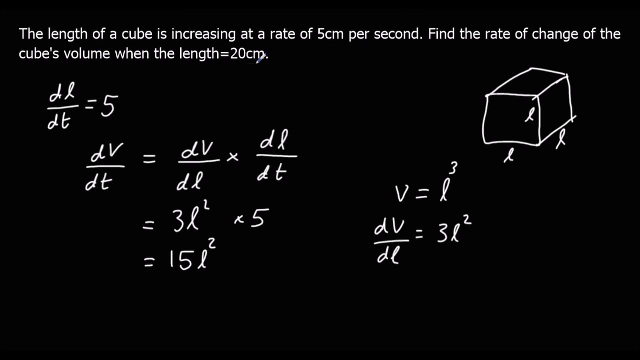 is going to be 3l squared, so times by the power. take one off the power: dvdl 3l squared. so that means dvdt is 3l squared times 5 or 15 l squared. and we wanted to know the volume when l is 20. so when l is 20. 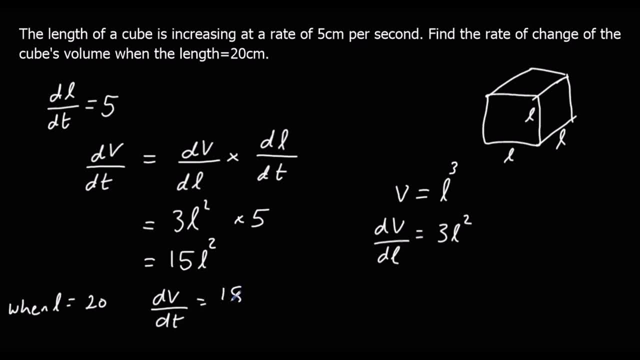 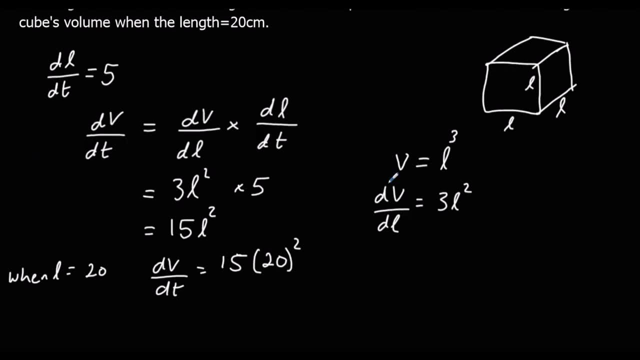 the vdt is 15 times 20 squared, so 15 times 400, which is going to be 6000. so it's dvdt. so the units again, we were measuring in centimeters, so volume, centimeters cubed. so the rate of change of volume is centimeters cubed per second. 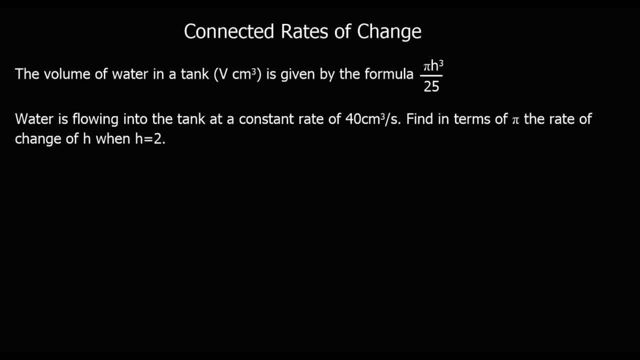 okay, here's another question. so we've got the rate of change of volume is centimeters cubed per second. so the rate of change of volume is centimeters cubed per second. So we've got the volume of water in a tank is given by the formula pi, H cubed over 25.. 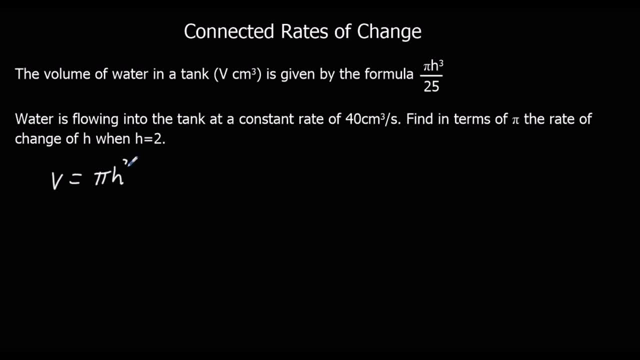 So we'll write: V equals pi, H cubed over 25.. Water is flowing into the tank at a constant rate of 40 centimetres cubed per second. So that is. so we've got volume centimetres cubed. So dV, dt is the rate of change of the volume, and that is 40.. 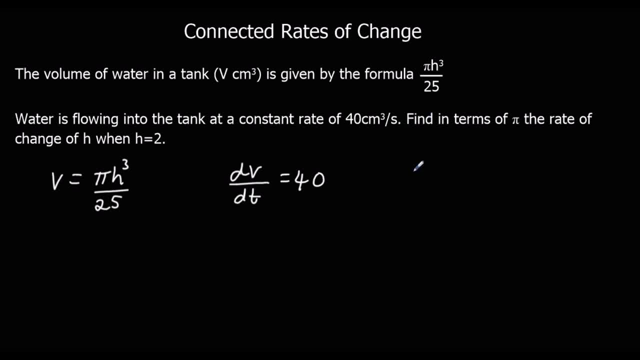 So every second the volume of water increases by 40. So dV dt is 40. So we want the rate of change of H when H is 2. The H dt, the rate of change of H, is the H dt. 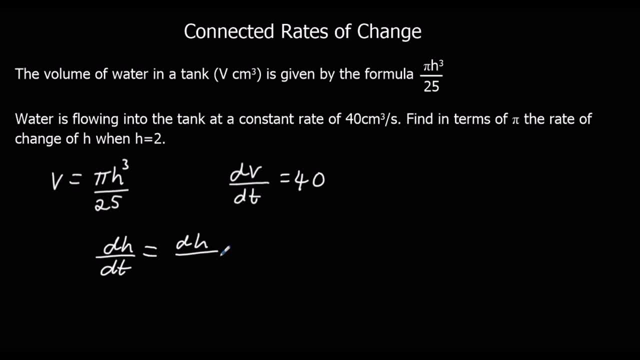 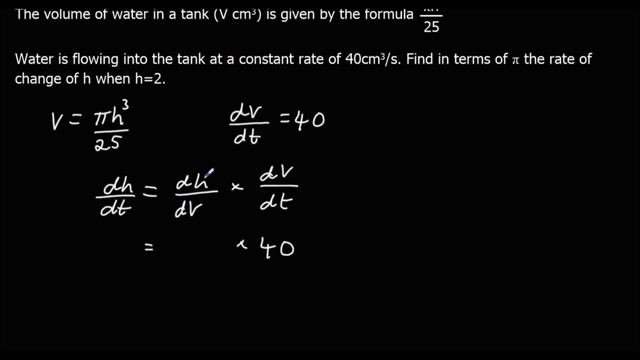 And that's 40.. That'll be dH d-something times d-something dt. Our other variable is V this time. So we know dV dt. We don't know dH dV. yet dV dt is going to be 40, and we're going to times it by dH dV. 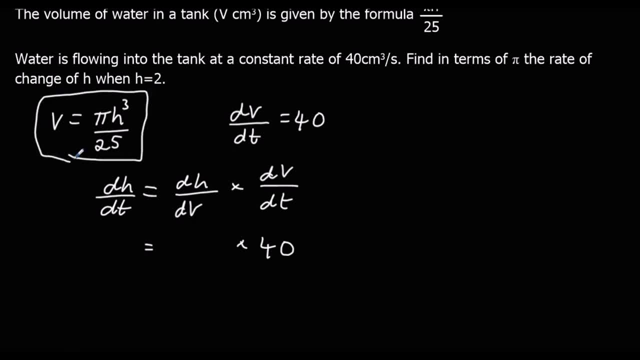 We've got a formula linking V and H, so we'll use that. We're going to do dV dH. We can do that, and we'll flip it over afterwards to get dH dV. That's not a problem. 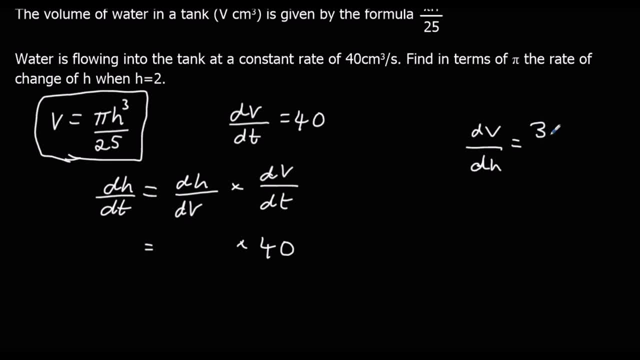 So dV, dH. we're going to times by the power. So 3 pi H squared, take one off the power. So that's our dV, dH, dH, dV is going to be the same thing flipped over. 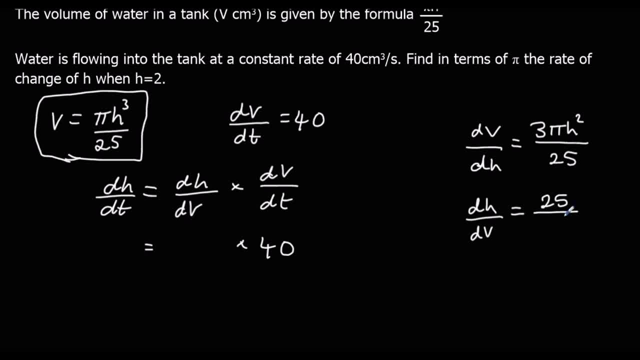 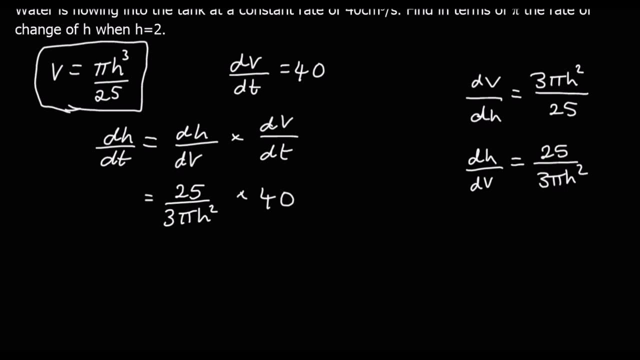 so we're going to flip it over. so 25 over 3 pi h squared, so that's dhdv. so we'll substitute it in here: 25 over 3 pi h squared, okay, so we'll simplify this a bit. so if we do 25 times 40, 25 times 4 is. 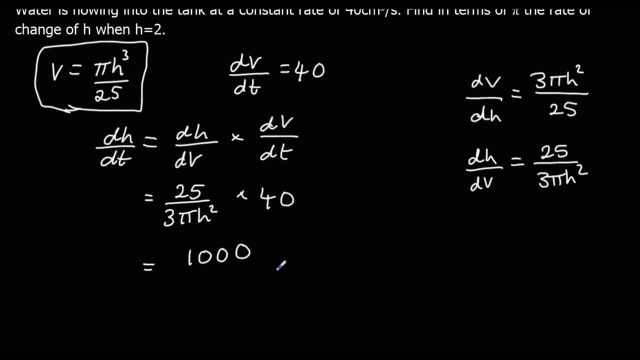 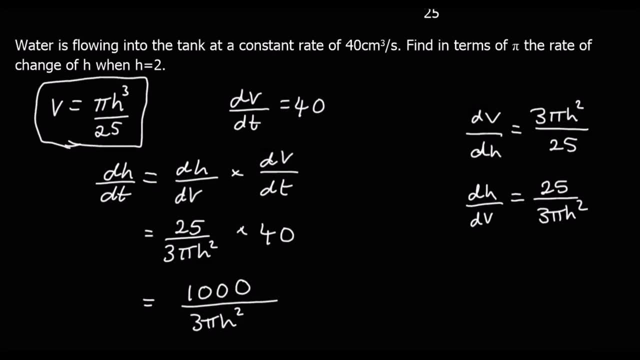 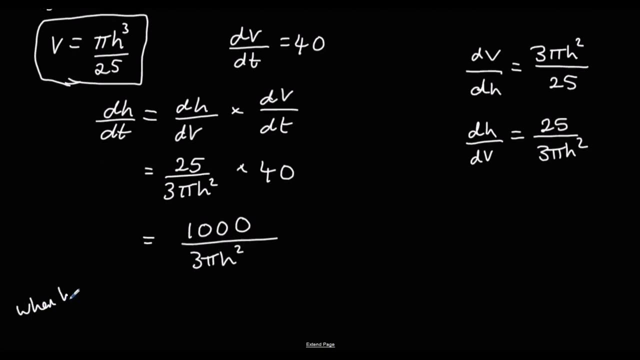 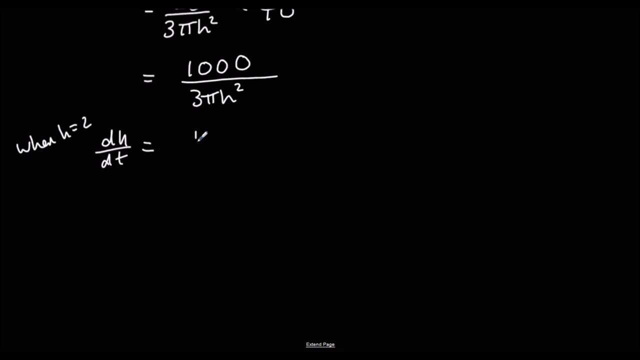 100, so that'll be a thousand over 3 pi h squared. and we want to know dhdt when h is 2, so when h equals 2, dhdt is 1000 over 3 pi times 2, so that'll be a thousand over 3 pi h squared. and we want to know dhdt when h is 2, so when h equals. 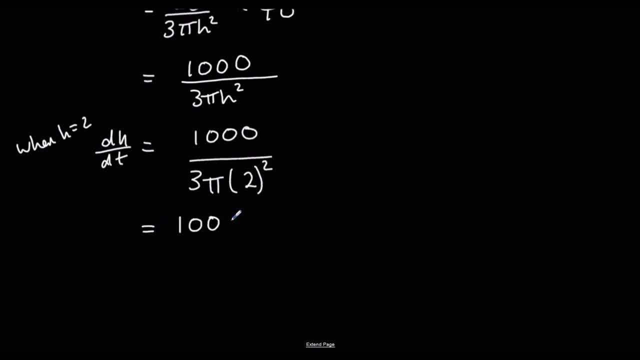 squared, so a thousand over, or 3 times 4, that's going to be 12. so a thousand over 12 pi. we can divide top and bottom by 4, giving us 250 over 3 pi, and that's in its simplest form. what are the units? so we're going to be measuring the. 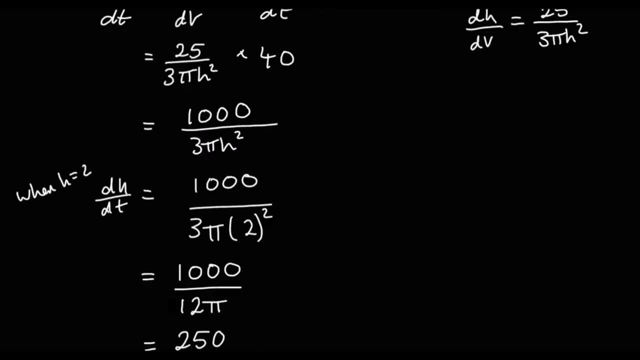 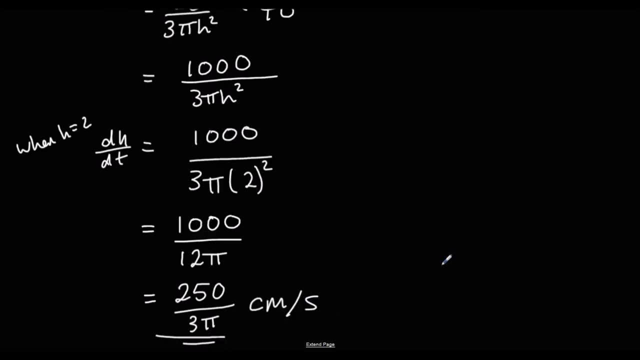 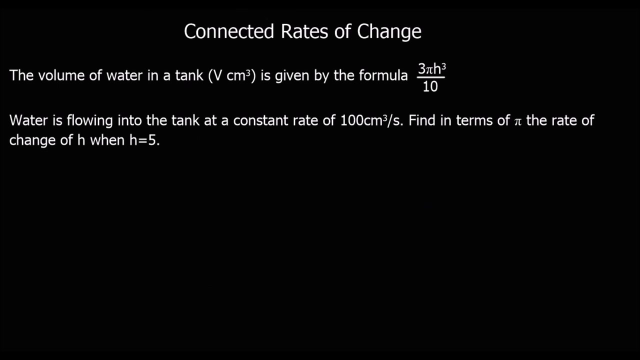 height in centimeters and centimeters. the rate of change of height is in centimeters per second, dh, so centimeters h over t, h over t, centimeters per second. okay, one more question. pause the video, give it a go and then press play when you're ready to go through. 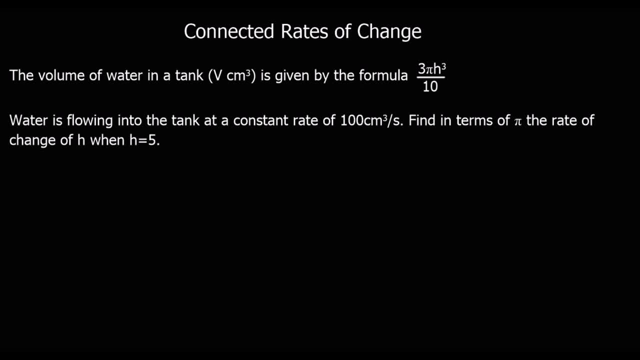 okay. so water is flowing into the tank at a constant rate of 100 centimeters cubes per second. so that's the rate of change of the volume. we know it's volume because it's in centimeters cubes, so the vdt is 100. we want to find out the rate of change of h, so we want dhdt. 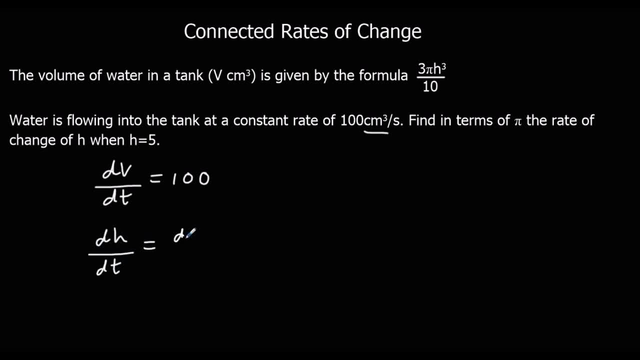 so we want dhdt, and that would be dhdt over pi. i squared so the rate of change of h. so we want dhdt, dH, d-something times, d-something dt, And our other variable is v. so we're going to fill in these with dv's.